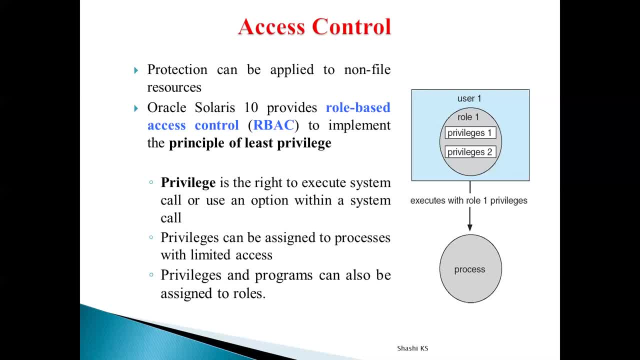 about how access control can be implemented, for how access control is implemented for non-file resources also. So one such example is: we are taking an example of the Solaris 10 operating system. We are taking an example of the Solaris 10 operating system. We are 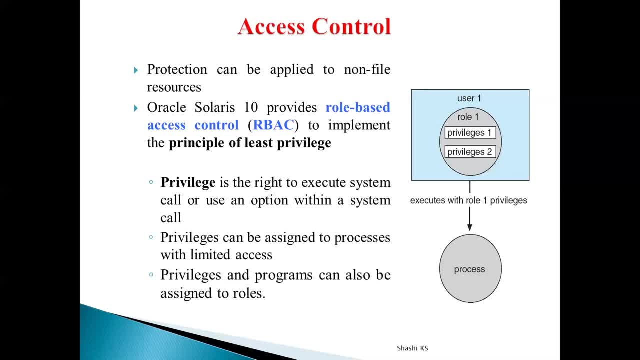 taking an example of the Solaris 10 operating system, which was developed by Sun Microsystems. So in this Solaris 10 operating system, it makes use of the principle of least privileges and, with the help of principle of least privileges, it implements role-based access control. Just. 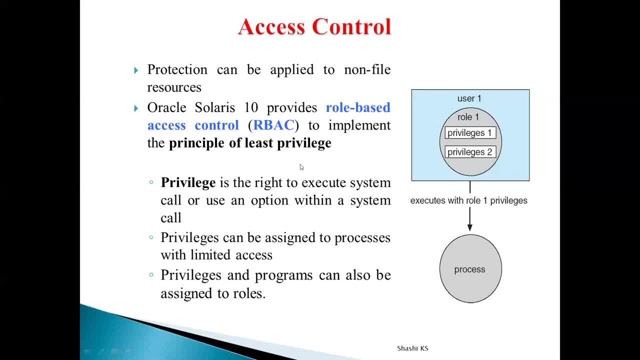 try to recall what we learned in the principle of least privileges. So what does the principle of least privileges say? The principle of least privileges says that whatever may be the systems or the processes or the processes that are involved in the system, the system or the processes or the programs residing in the computer system just give just enough. 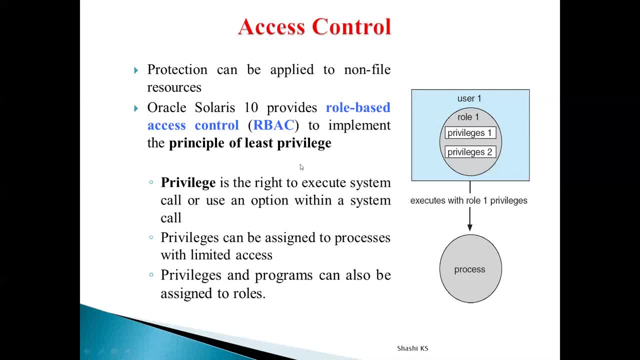 privileges for these processes to complete their tasks. The program or the processes should be given only just enough privileges to complete their tasks. That is the principle of least privilege. So that is being extended in this Solaris 10 operating system to provide role-based access control. We call it in short as RBAC. So here, what is the meaning of privilege? 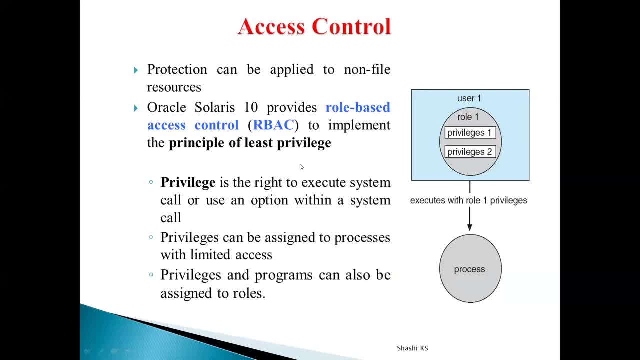 Yes. first of all, let us try to understand what is the meaning of privilege. Privilege is nothing but the right to execute a system call. What I mean by privilege is the right to execute a system call, Say, for example, If a process wants to open a file or do want. 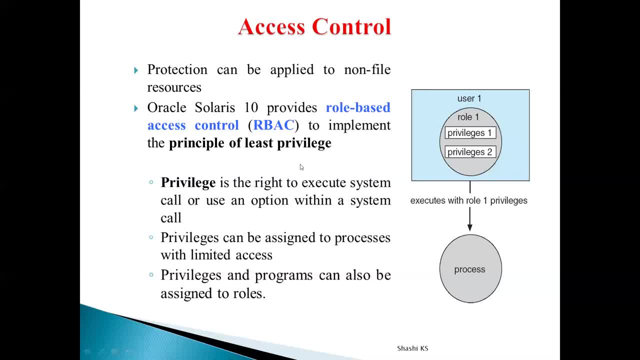 to do a read operation on the file, it should have the right to execute, to execute that system call. So that right to execute a system call is called us privilege or privilege. We can also say an option within a system call, Right to execute an option within the system call is 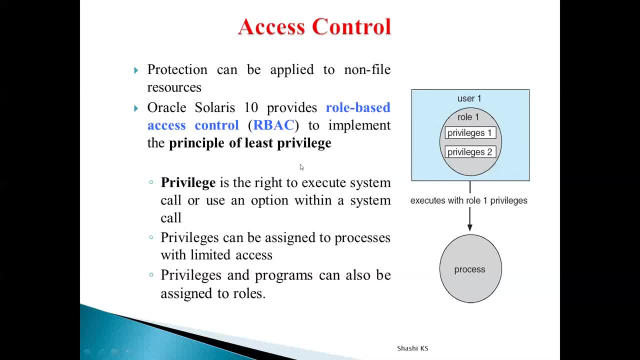 system call may also be called as privilege Say. for example, if I want to issue the open system call, then I want to. I may want to use the open system call with read access or with read write access, that the read and write are called options within the open system call. So I may want to use 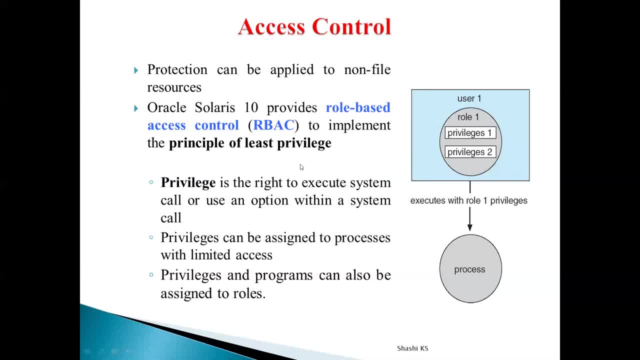 the. I may want to use the read and write operations within the open system call. So that is also called as a privilege, So you can assign privileges to processes. So. so how are we going to assign privileges to processes? There are two ways by which we can make use of this privilege. 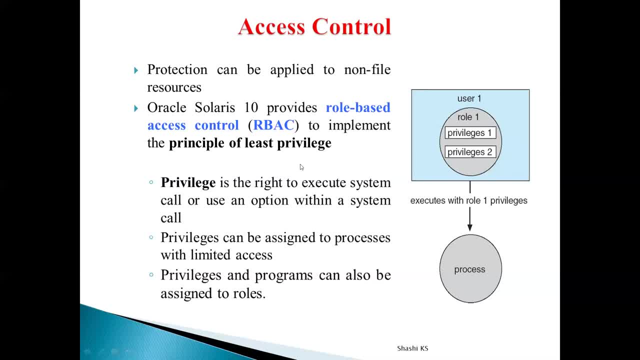 concept One is: you can make, you assign this, privileges to processes, And the other one is: privileges can be assigned to roles. Okay, When, when you assign privileges to processes, then you can assign them and then you can limit them to only that particular. 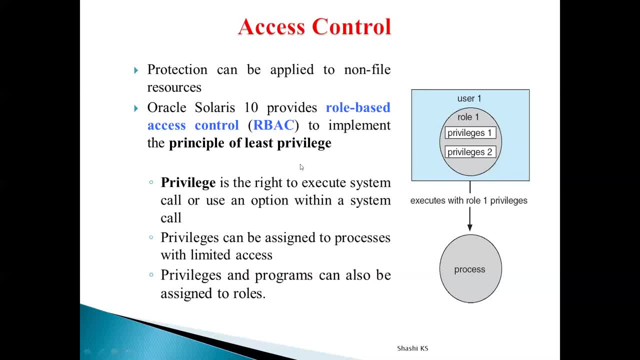 you can give them only the access which they require to complete that task. Do not give them more access than what is required for them. So just assign privileges to processes and then give them the privileges to processes. So that is how you can make use of this privilege concept. 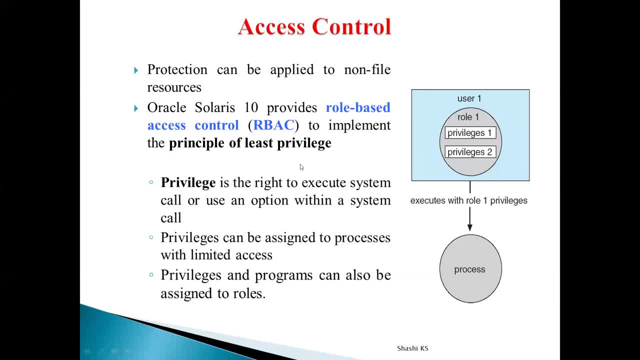 them limited access, so that they are, they are just given only the access which they require to complete their task. for example, if you have a computer operator or the system operator whose job is to copy all the backup files from the file system, then just to give him access to only those. 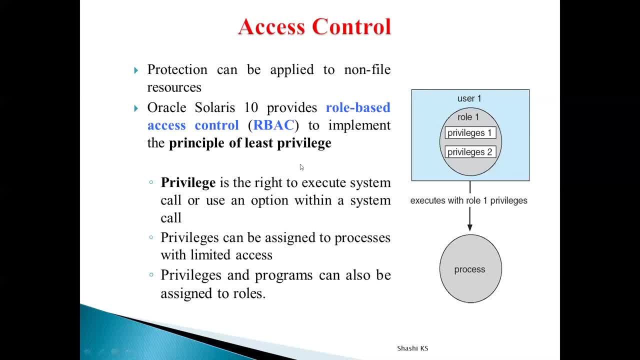 commands required for doing the backup operation and just give him access to only the files which he has to do the backup which he requires to do the backup operation. that is the meaning of giving privileges to processes and then giving them only limited access, to giving them limited access. 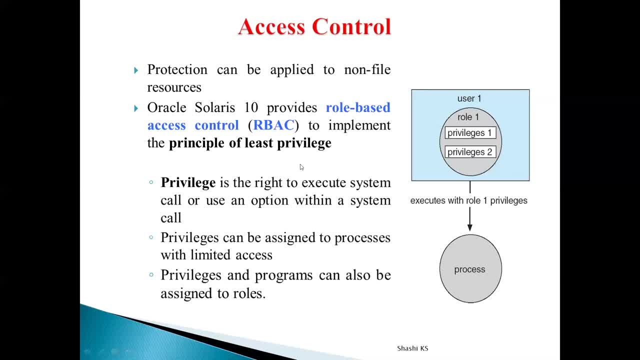 so the other way is: you can assign privileges to roles. now, what is the meaning of roles? privileges can be assigned to roles and users. if they want to perform a task, then they will take up a role which will enable a privilege for them. okay, the second method, which is called as role based access. 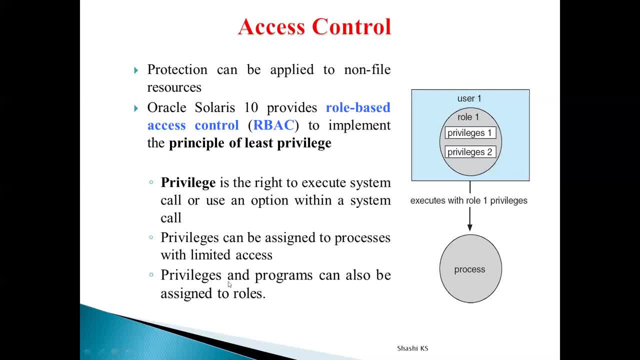 control is nothing but privilege is nothing but the right to execute something, system called okay. so you are saying this privileges to roles and if a user or a process wants to, wants some privilege to execute a task, he will take up the role. how will he take up the role? 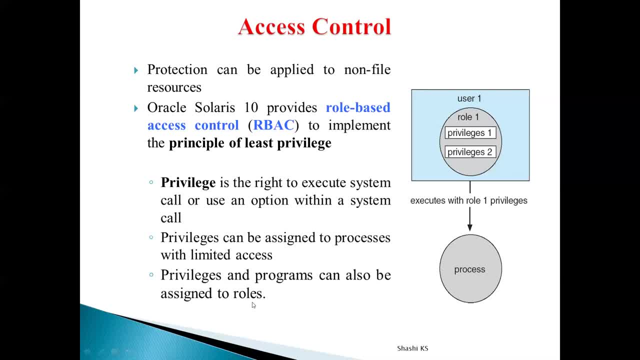 he'll have to. he may have to specify the password for the role. so he will specify the password for the role and he will take up the role and by taking up the role he will get the privilege to execute the task and then he will complete the task. so that is that concept of role-based access. 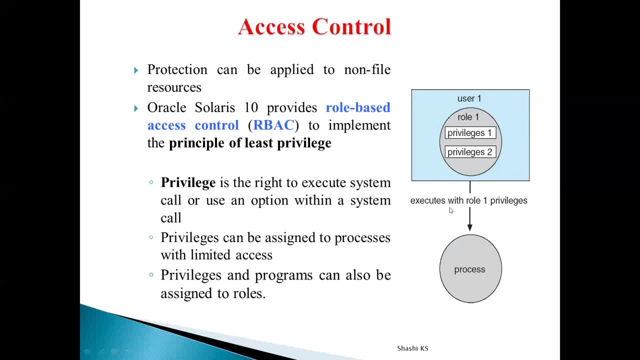 control is being represented in this diagram. you can see here that you have role one which gives a user privileges- privilege one and privilege two. okay, if the user one wants to execute a process with privileges- privilege one and privilege two. if the user one wants privilege one and privilege two,